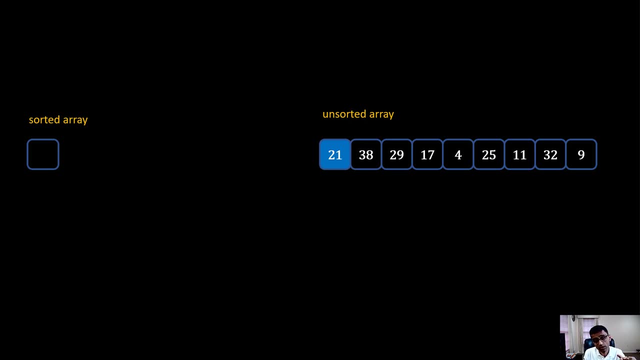 such a way that that array remains sorted. Right now there are no elements, so you can just put the element directly there. Let's take the second element 38. you want to put in that array so that that array remains sorted. So you will. 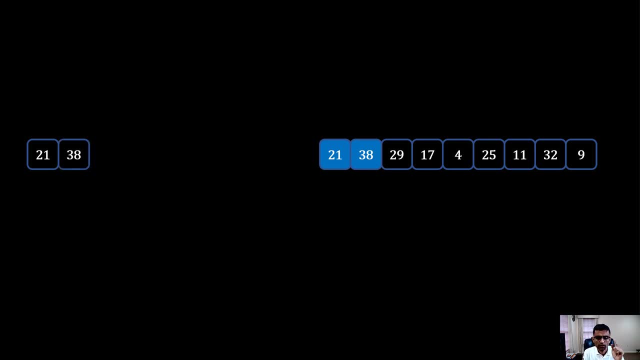 put 38 after 21.. Then you pick 29.. Now when you put 29 into that array, you cannot put it at the end because it has to be after 29 before 38. so you'll have to do little bit array shuffling here and then insert it in the middle. so 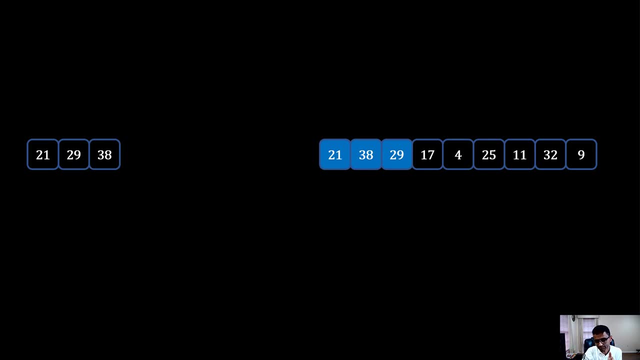 you are moving 38, one element behind. next comes 17 for 17. you will put that into the first place. so you take 17 from unsorted array. compare it with the elements starting from beginning in the sorted array. when you compare it with 21. 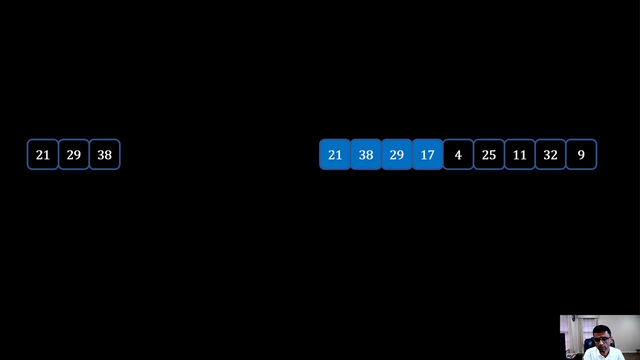 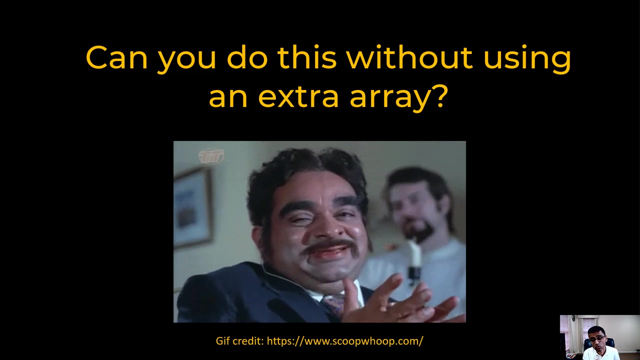 you find that 21 is already greater, so then you just put it in the front. so you continue this way and on the left hand side you will get a sorted array. this approach is fine, but it requires using separate array. the question is: can you do it without using a separate array? so just pause the video. think about this. 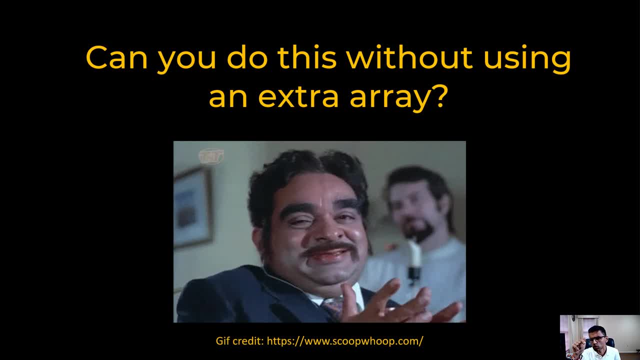 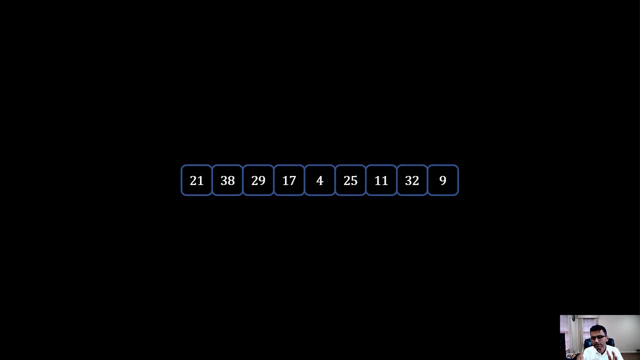 I think there is a way you can. you use it. you can do this from the same array itself, so that you don't have to create an extra array. all right, let's talk about that approach. I hope during that pause you get an idea. see the way you learn algorithms is before looking at the 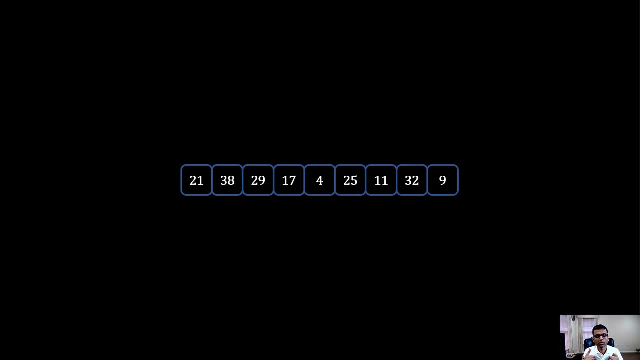 solution directly. you try to come up with your own idea on how you can solve a problem. that will make your very good programmer, that will make your algorithms trigger skills very, very strong. so now I have this array, so I take a pointer. I start from the second. 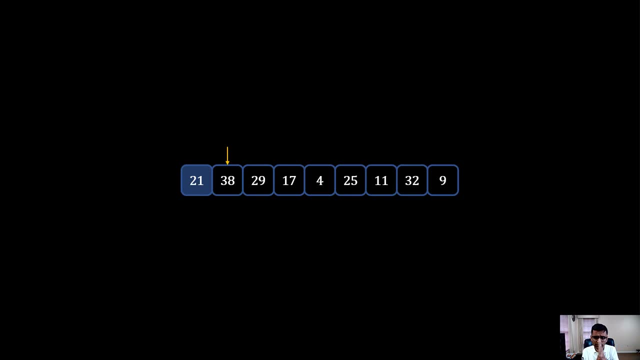 element. so anything to the left hand side of the pointer is a sorted array. when I start with second element, the first element is of course a sorted because if you have one element array it is sorted all the time. now you take the second element and you try to put in on the left hand side so that it is sorted. 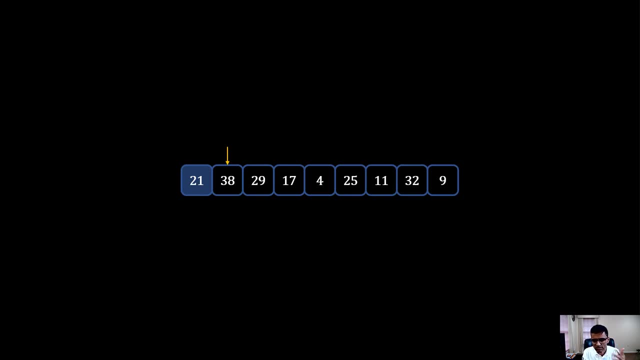 so left hand side, it's 21, which is less so already sorted. so let's move the pointer. okay, when you move the pointer, I am changing the color of this 38 cell, which means now the first two elements are sorted. I go to 29 now. I compare it. 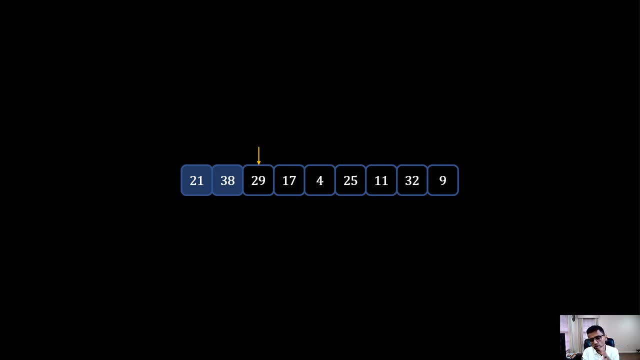 with the sorted array so that then I go to 38 first, then 38 is bigger. okay, so then I go to 21. 21 is smaller, which means I need to 29 in between 21 and 38. so I will do that and we'll look into. 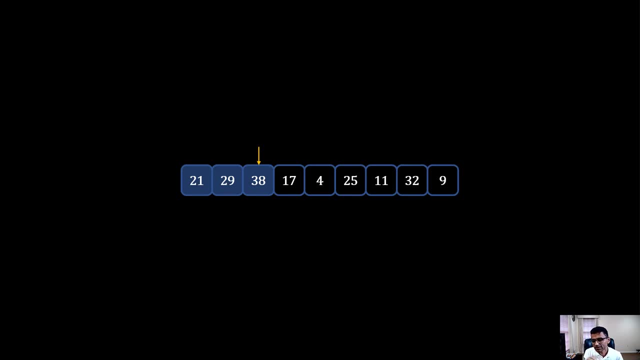 Python code how exactly to do this. but in this theory part, just assume that you're picking up element from unsorted array, putting it in a sorted array so that the order is maintained. you move to 17. then you look in the left hand side so you begin with 38 first. 38 is bigger. 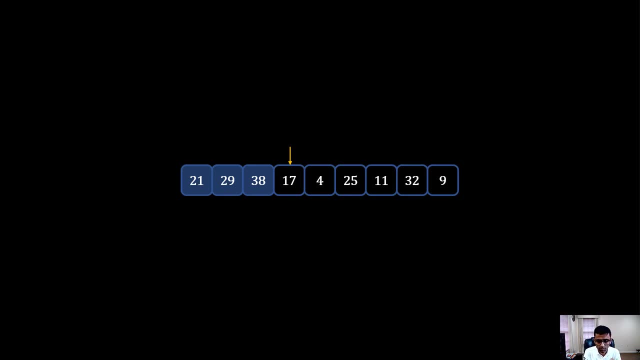 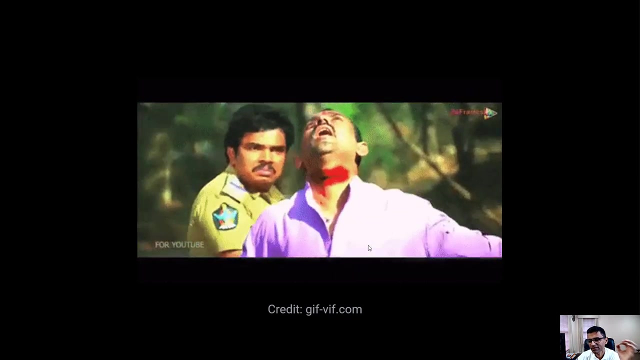 okay, you move to 29 bigger, move to 21 bigger. you insert 17 at the beginning. so this is how now this looks, and you keep on doing this until your entire array sorted. so you see how a simple trick can kill so many birds in one storm. 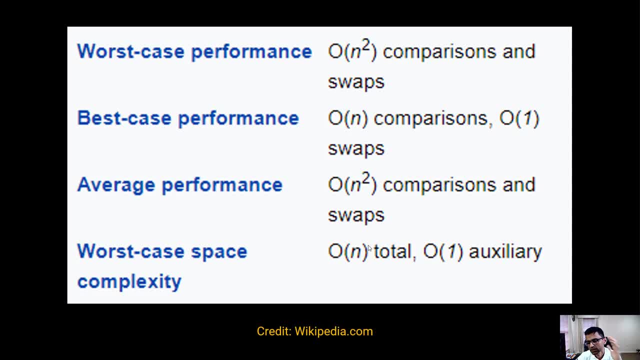 all right, let's talk about the performance. i took this from wikipedia. the worst case performance is order of n, square, comparison and swaps. so just imagine the whole array is not sorted. so every time you pick up the element, you have to perform those many swaps. so you are going. 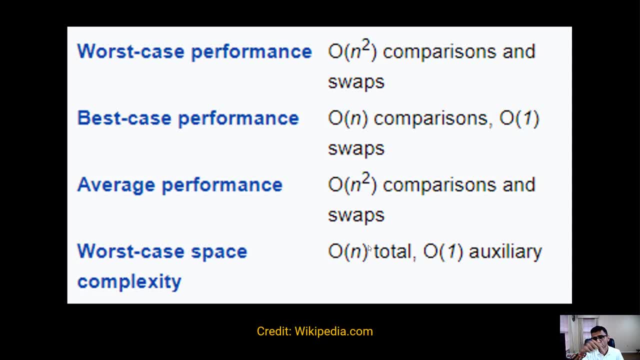 through n elements and for every element you are doing n swaps. that's why order of n- square base case is order of n, because even if the array is sorted, you are still doing n comparison and swaps will be order of one. the space complexity: there is not much space complexity. 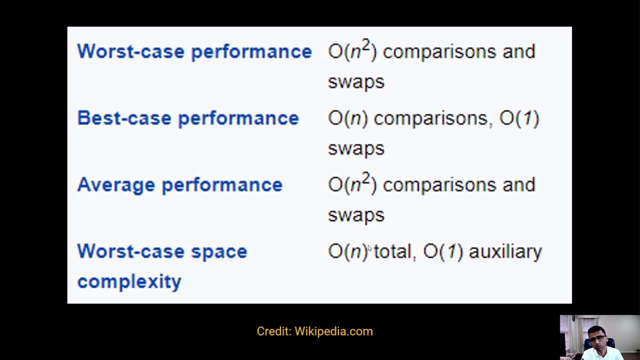 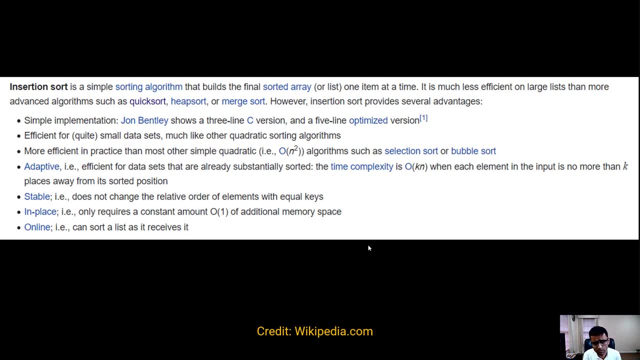 maximum order of one, because you might create one variable to hold that anchor element. all right, again, this is from wikipedia. it's a simple algorithm. you will see in python it's only few line of code, but when your list is very big it is not efficient. so you will use this for maybe smaller list, and here are some of the benefits you can read through: 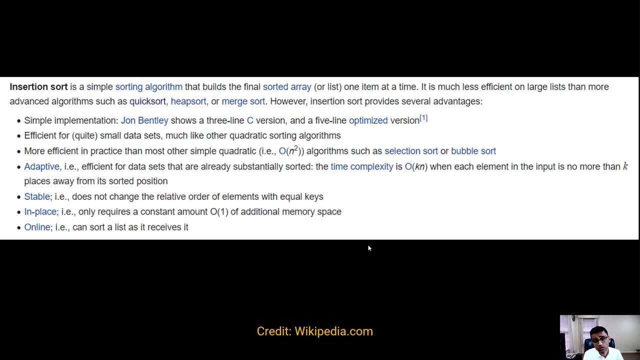 them: uh benefits and some of the aspects of insert and sort. when you use sort function in python, it already uses some internal- uh some algorithm, so you will never have to more. in most of the cases when you're doing python programming, you don't have to do inserts and sort implementation on your own. you're using this inbuilt algorithm. 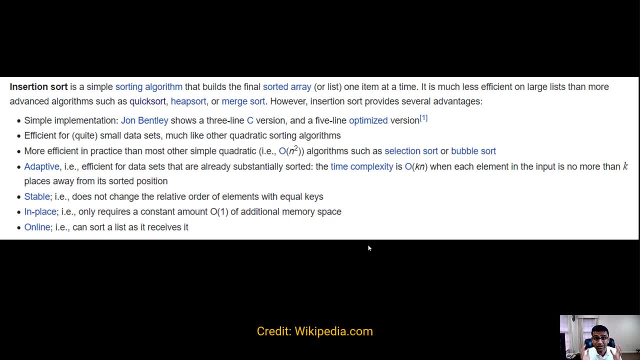 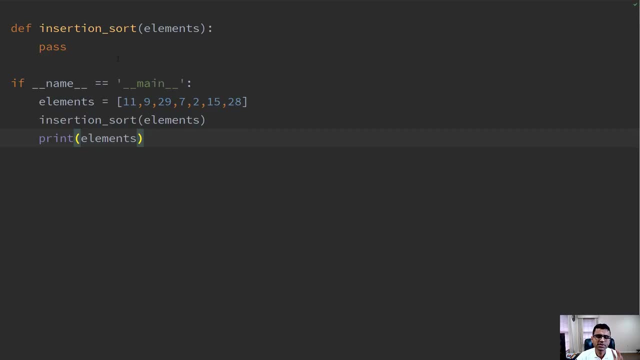 but having this understanding of how algorithm works allows you to develop this algorithmic mindset and you might use the things which you learn from this to make your code better. let's jump into coding now. let's start with the presentation. we always start with the first element. 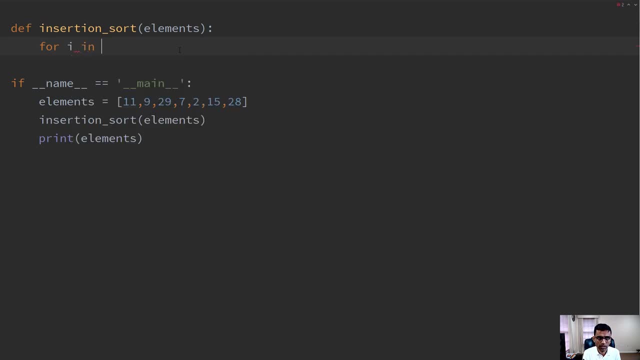 so we'll run a loop where we'll say, for i in range one, two length of elements. okay, do something. we saw that. the first element, you can consider it as sorted, then start with the second element and then, uh, try to take one element at a time and try to put it in the sorted area on the left hand side, in a right 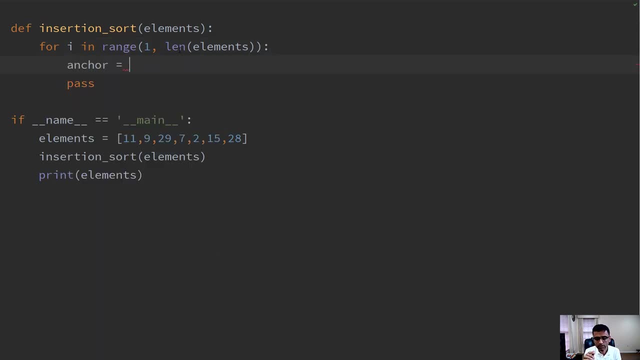 order. so we'll call the element that we are dealing with right now an anchor. so your anchor is elements of i and what you're doing is you're going on the left hand side. so left hand side is what. left hand side is, um element which is. 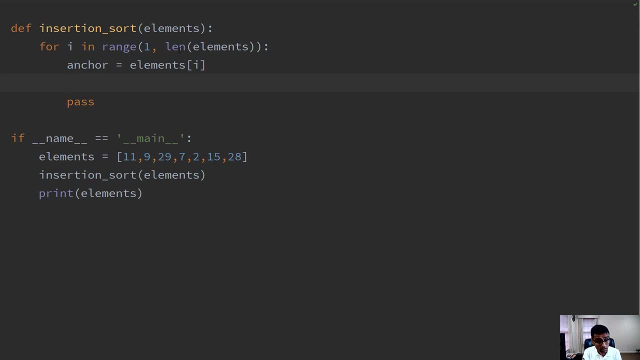 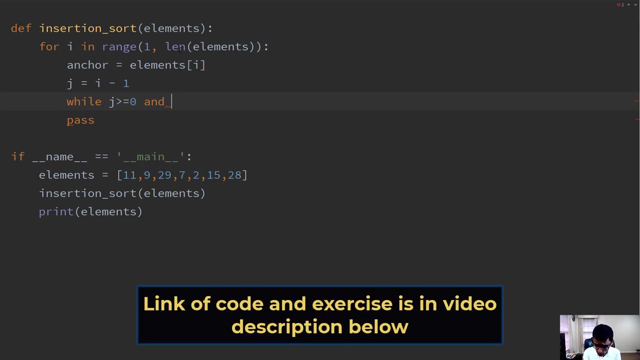 one place less than the current element, so let's call it j. j is one less than your current element, right? so i minus one, and you want to start from that to all the way till zero. so, while j is greater than equal to zero and you want to stop so, until so, let's do this. 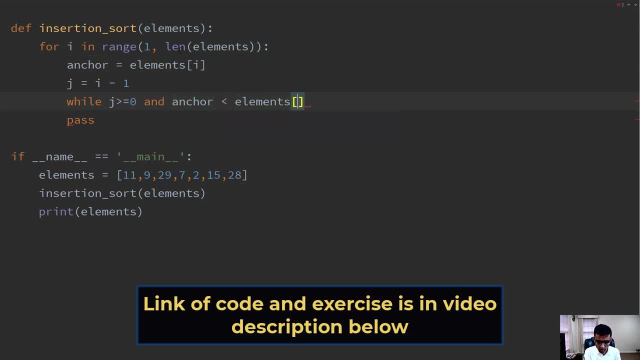 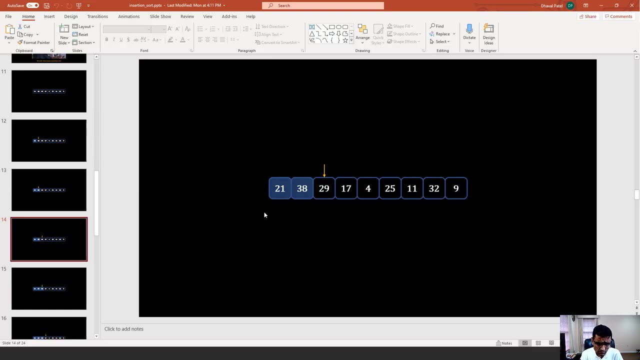 until your elements of j are greater than anchor, you continue. but right, and then when you continue, you want to swap those elements. so you see this case here, here, uh, so here, uh, let's see. yeah, when you're at 17, you start with: okay, let's see, let's see. 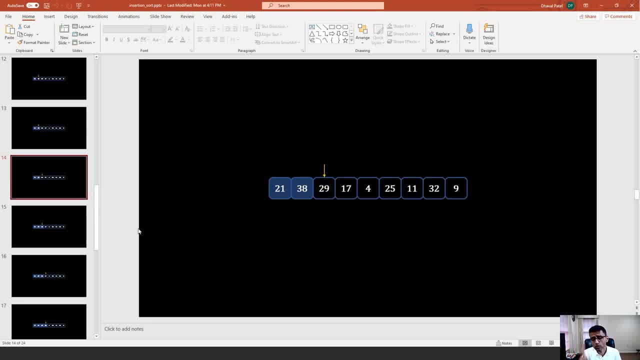 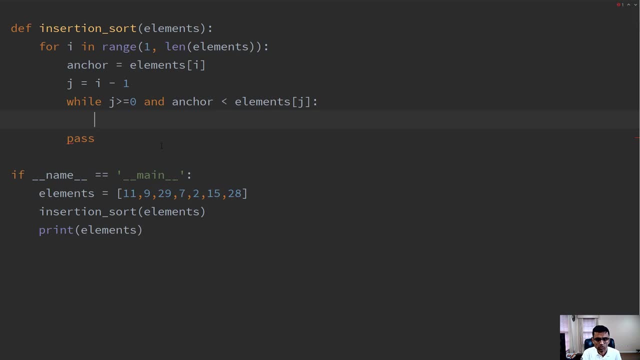 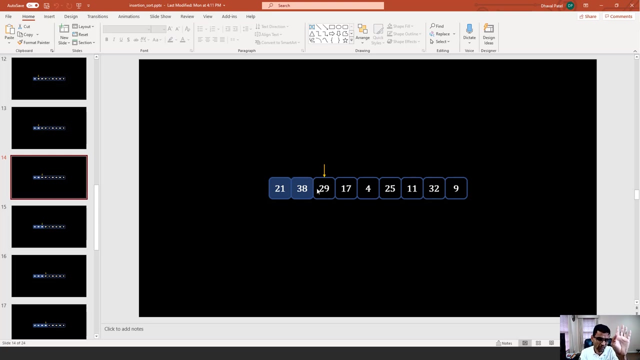 okay, let's see, let's do this. okay, when you are 29, you start with 38. 38 is greater. so you continue, you get 21. when you get 21, you stop okay and you make an exchange. so, and by the way, when you're here, what you'll do is you store 29 less in an anchor. 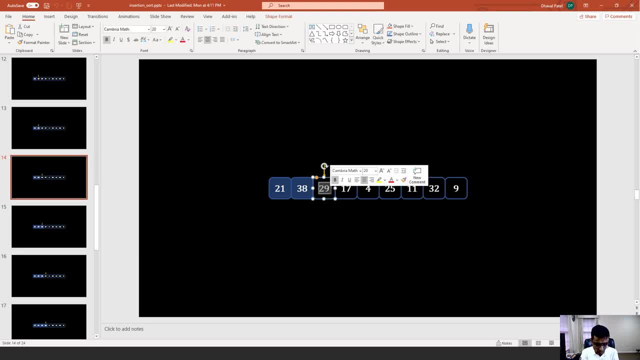 and then you swap 38 here, okay. so literally what you're doing is 29 is here, so this is your anchor now, okay, and then you put 38 here. you see, you put 38 here, then you go to 21, so 21 is greater than this, so you stop, okay, and then what you do is the anchor. 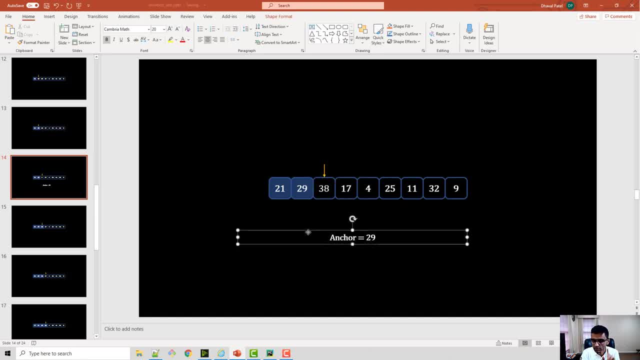 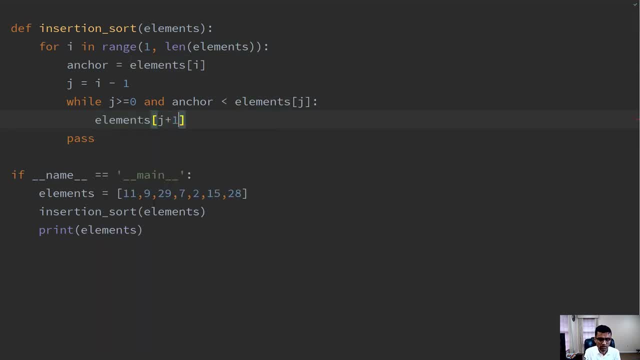 which is 29 you put here. so that's the method. so first we are doing swap, so in j plus 1 we are copying element from the left. so this is just swapping from left to right. of course you need to reduce j and then in the end you will do.